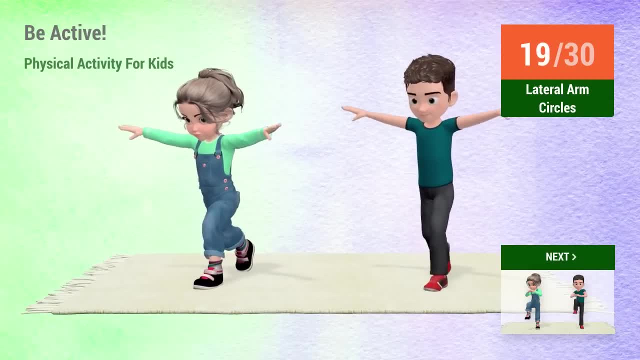 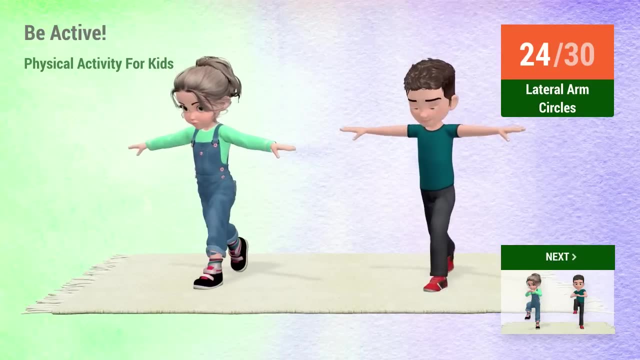 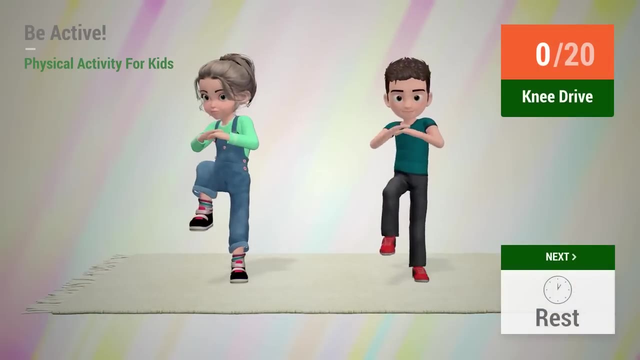 17,, 18,, 19,, 20,, 21,, 22,, 23,, 24,, 25,, 26,, 27,, 28,, 29,, 30.. Up next knee drive In 5,, 4,, 3,, 2, 1, go. 1,, 2,, 3,, 4,, 5,, 6,, 7,, 8,, 9,, 10,, 11,, 12,, 13,, 14,, 15,, 16,, 17,, 18,, 19,, 20,, 21,, 22,, 23,, 24,, 25,, 26,, 27,, 28,, 29,, 30. 1,, 2,, 3,, 4,, 5,, 6,, 7,, 8,, 9,, 10,, 11,, 12,, 13,, 14,, 15,, 16,, 17,, 18,, 19, 20.. 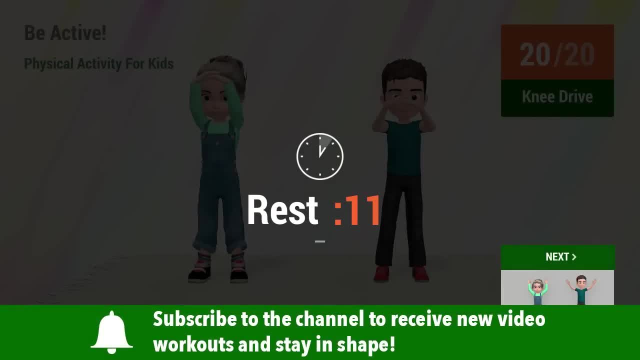 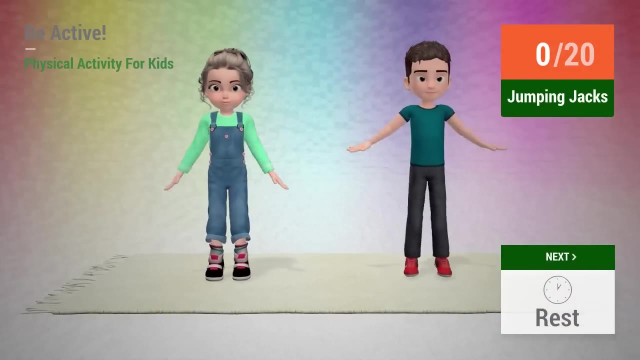 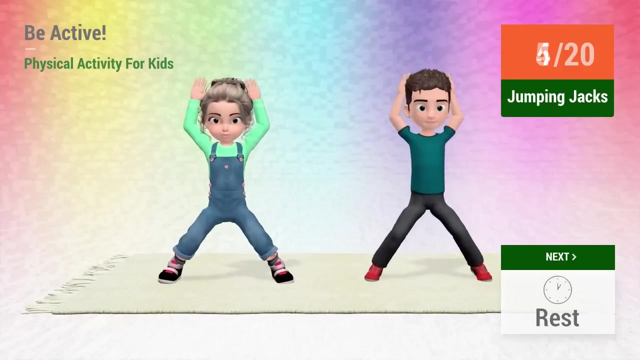 Rest time. Up next jumping jacks In 5,, 4,, 3,, 2,, 1, go 1,, 2,, 3,, 4,, 5,, 6,, 7,, 8,, 9,, 10,, 11,, 12,, 13,, 14,, 15,, 16,, 18,, 19,, 20,, 21,, 22,, 23,, 24,, 25,, 26,, 27,, 28,, 29,, 30. 1,, 2,, 3,, 4,, 5,, 6,, 7,, 8,, 9,, 10,, 11,, 12,, 23,, 24,, 25,, 26,, 29,, 30.. 1,, 2,, 3,, 4,, 5,, 6,, 7,, 8,, 9,, 10,, 11,, 12,, 23,, 24,, 25,, 26,, 29,, 30.. 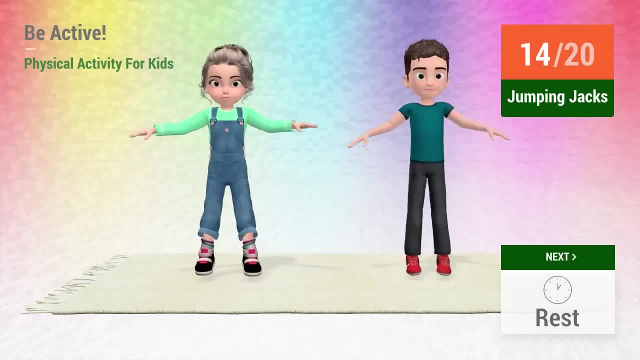 1,, 2,, 3,, 4,, 5,, 6,, 7,, 8,, 9,, 10,, 11,, 12,, 13,, 14,, 15,, 16,, 17,, 18,, 19, 20.. 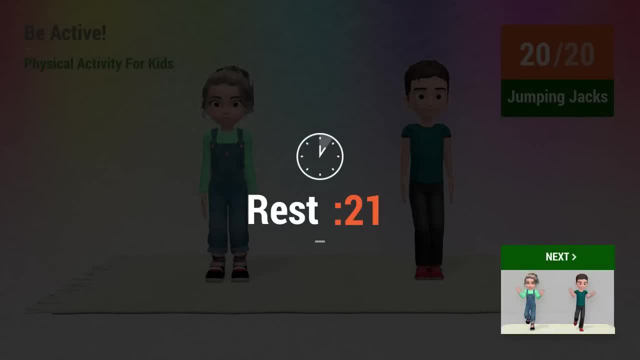 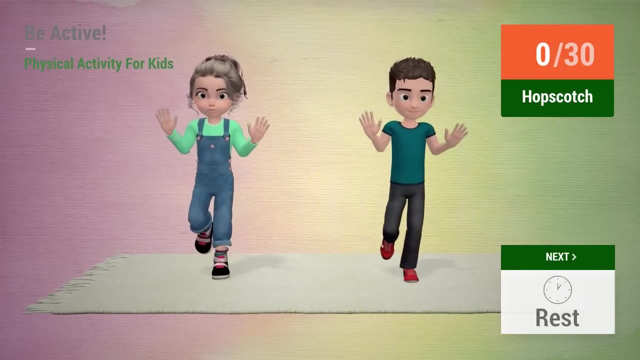 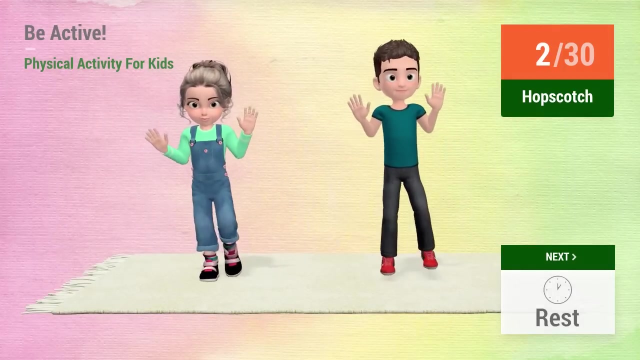 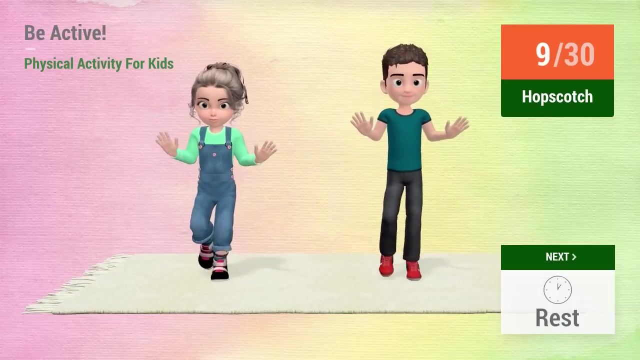 Rest time. Up next hopscotch In 5,, 4,, 3,, 2,, 1, go 1,, 2,, 3,, 4,, 5,, 6,, 7,, 8,, 9,, 10,, 11,, 12,, 13,, 14,, 15,, 16,, 17,, 18,, 19, 20.. 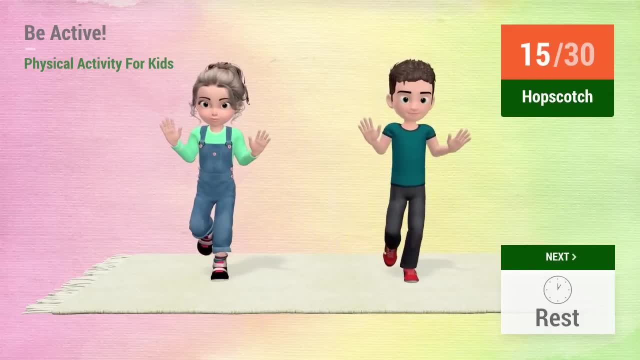 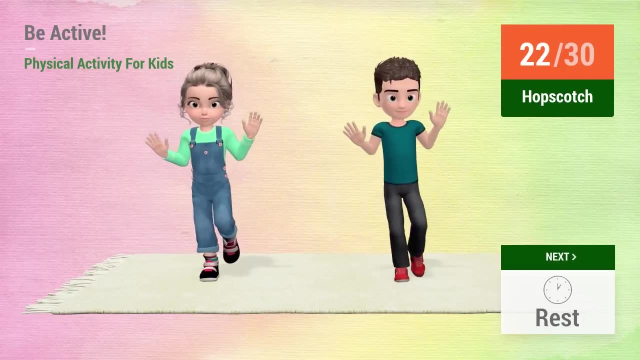 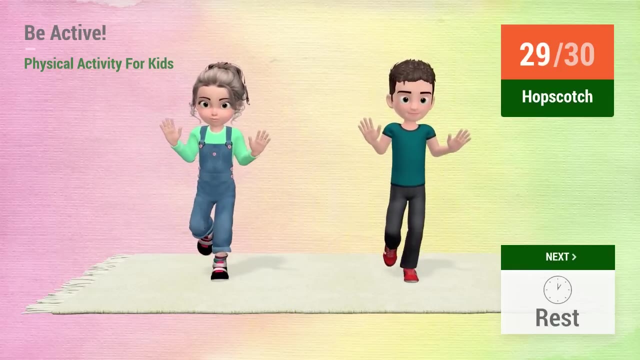 Rest time. Up next jumping jacks: 1,, 2,, 3,, 4,, 5,, 6,, 7,, 8,, 9,, 10,, 12,, 13,, 14,, 15,, 16,, 17,, 18,, 19,, 20,, 21,, 22,, 23,, 24,, 25,, 26,, 27,, 28,, 29,, 30. 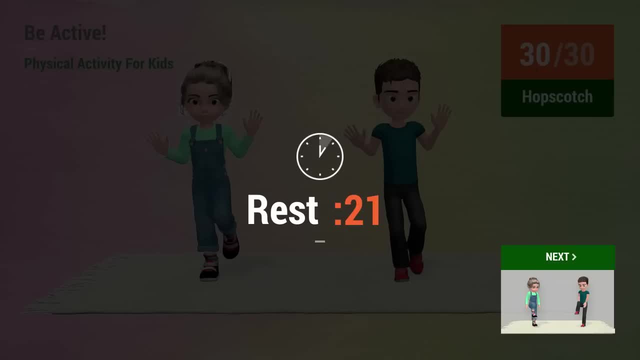 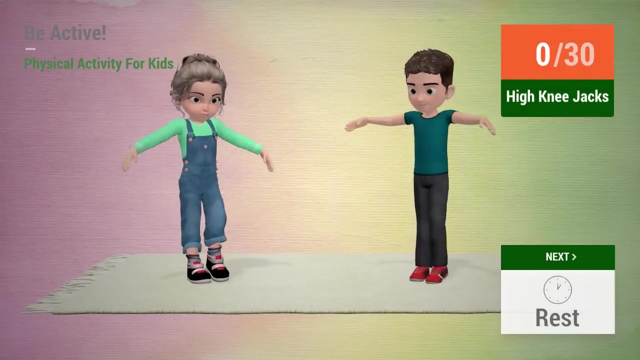 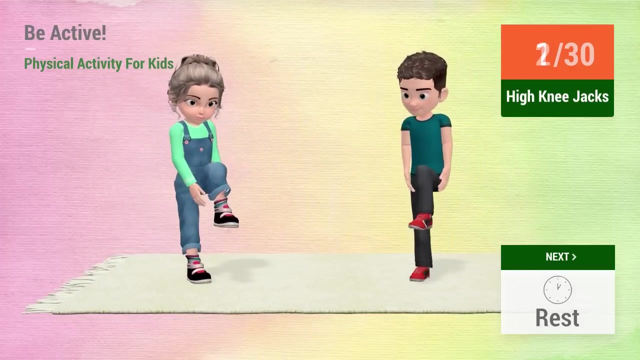 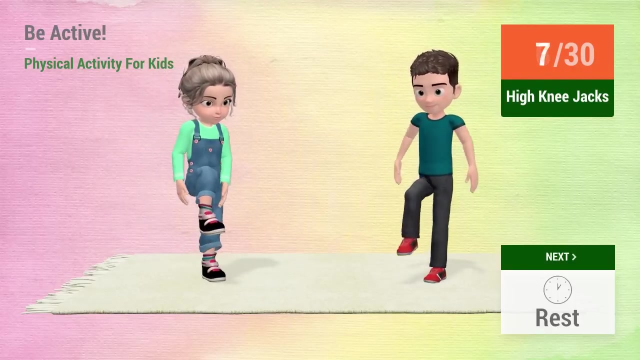 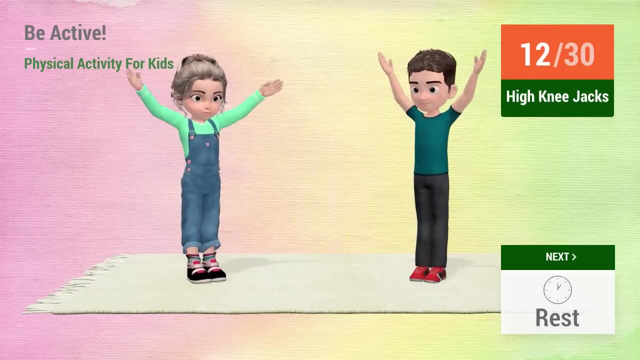 Rest time. Up next high knee jacks In 5,, 4,, 3,, 2, 1, go 1,, 2, 3, 4.. 1,, 2,, 3,, 4,, 5,, 6,, 7,, 8,, 9,, 10,, 11,, 12,, 13,, 14,, 15,, 16,, 17,, 18,, 19,, 20,, 21,, 22,, 23,, 24,, 25,, 26,, 27,, 28,, 29,, 30. 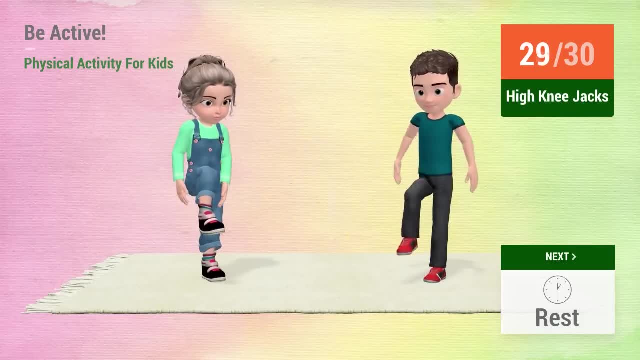 Rest time: 1,, 2,, 3,, 4,, 5,, 6,, 7,, 8,, 9,, 10,, 11,, 12,, 13,, 14,, 15,, 16,, 18,, 19,, 20,, 21,, 22,, 23,, 24,, 27,, 28,, 29,, 30. 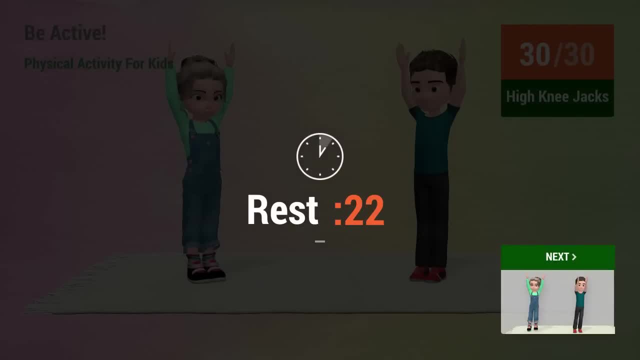 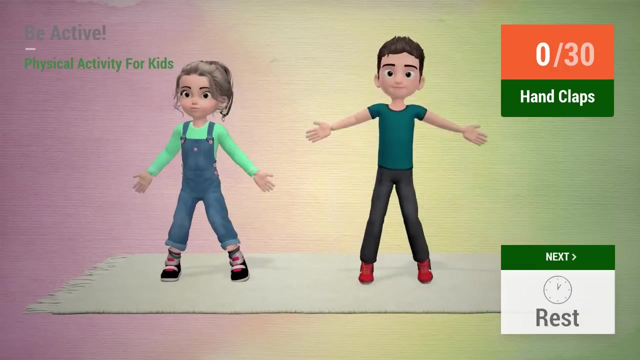 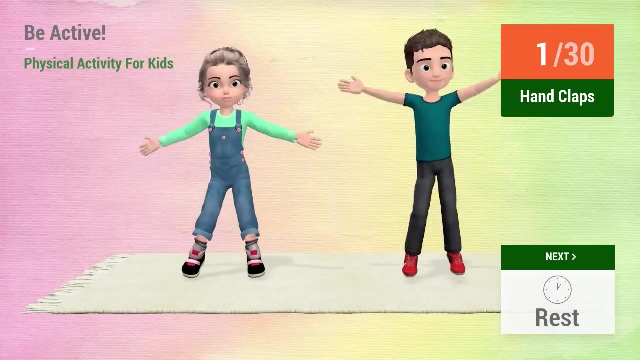 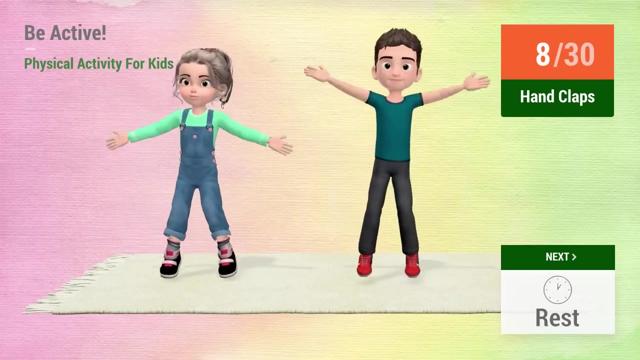 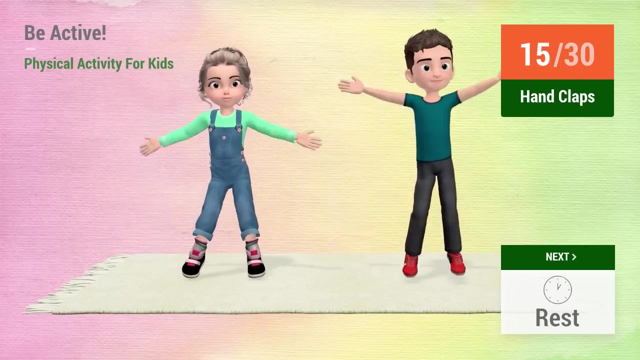 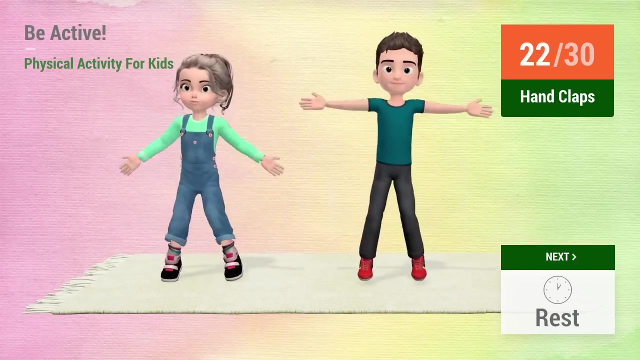 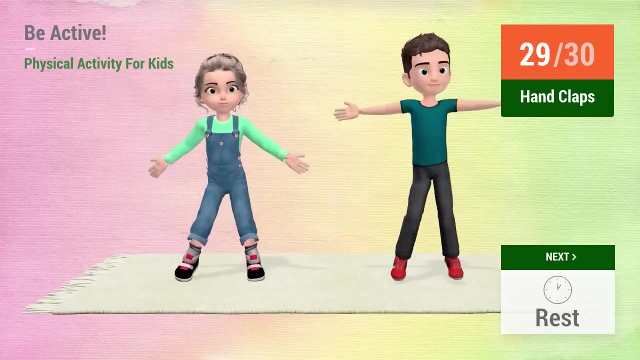 Rest time. Rest time up next hand claps in five, four, three, two. one go one, two, three, four, five, six, seven, eight, nine, 10, 11, 12, 13, 14, 15, 16, 17, 18, 19, 20, 21, 22, 23, 24, 25, 26, 27, 28, 29, 30 rest time. 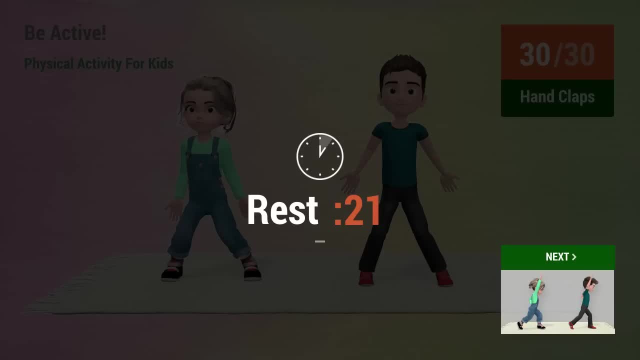 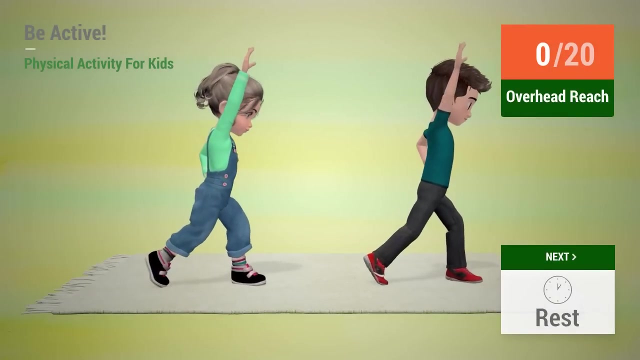 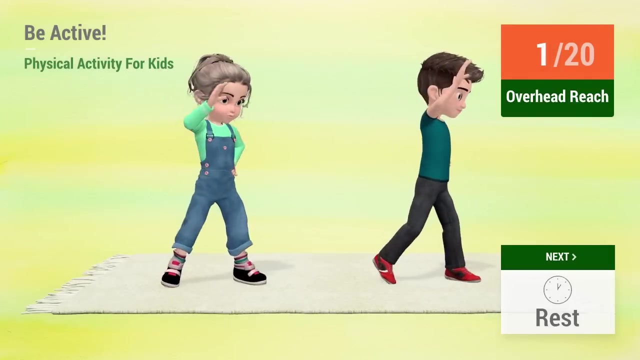 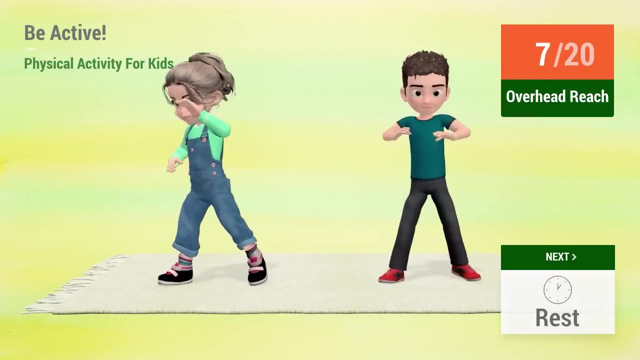 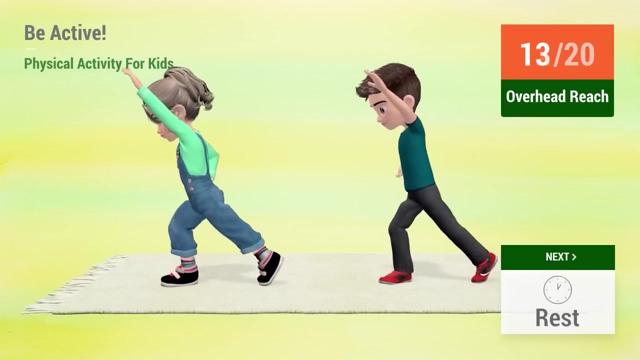 okay, now are you ready? up next overhead, reach in five, four, three, two. one. go one, two, three, four, five, six, seven, 8, 9, 10, 11, 12, 13, 14, 15, 16, 17, 18, 19, oh good, now 19,, 20, rest time. 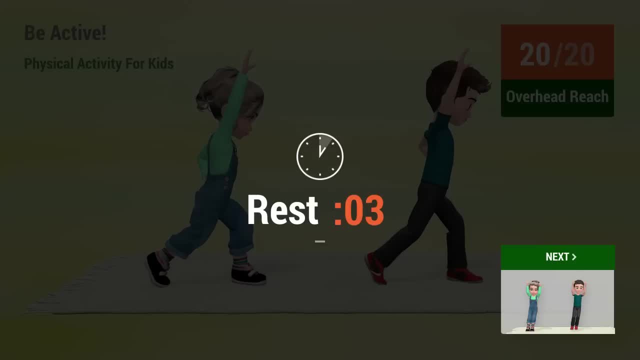 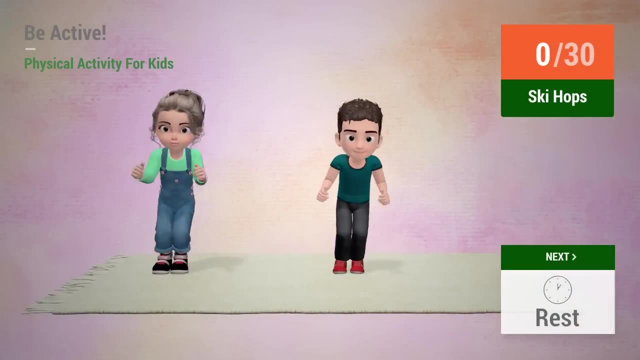 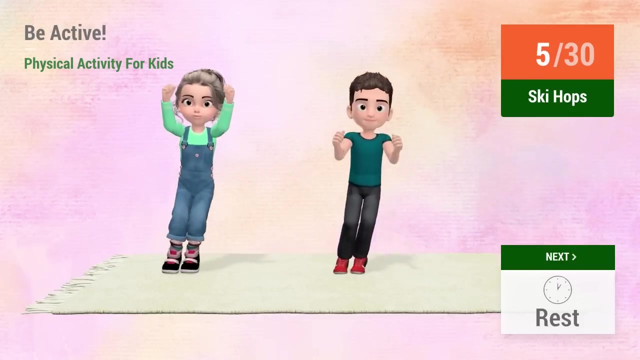 Up next ski hops In 5,, 4,, 3,, 2,, 1, go 1,, 2,, 3,, 4,, 5,, 6,, 7,, 8,, 9,, 10.. 11,, 12,, 13,, 14,, 15,, 16,, 17,, 18,, 19,, 20,, 21,, 22,, 23,, 24,, 25,, 26,, 27,, 28,, 29,, 30.. 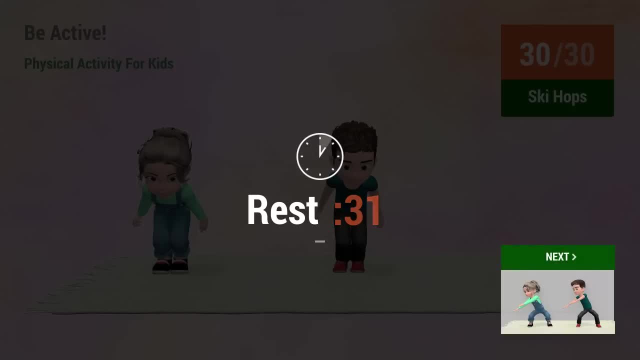 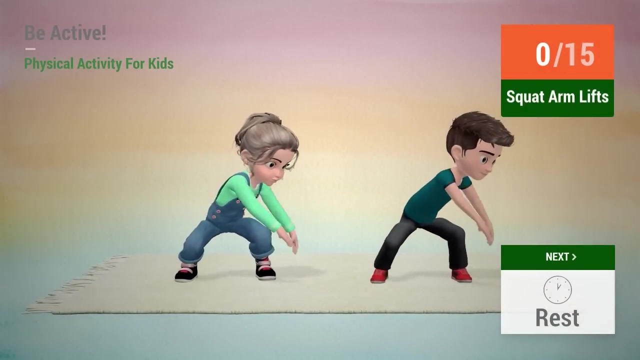 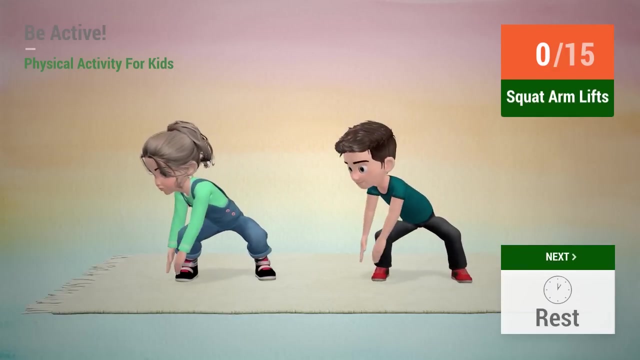 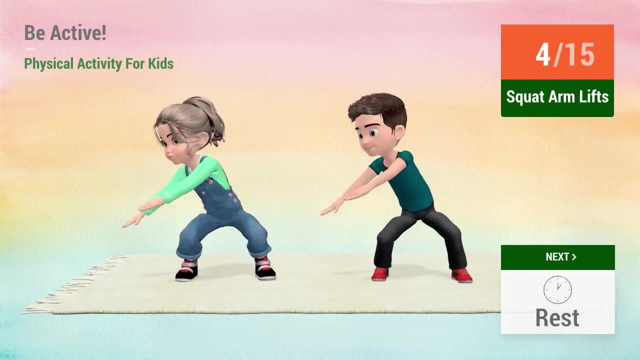 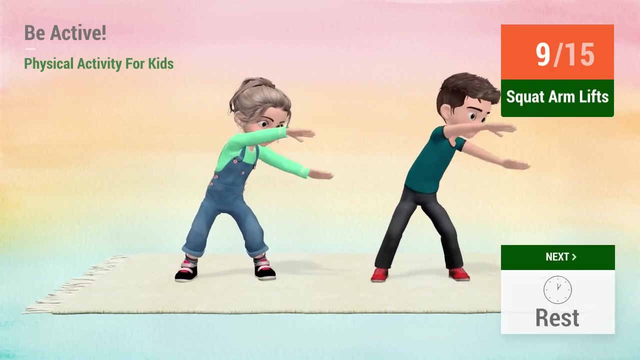 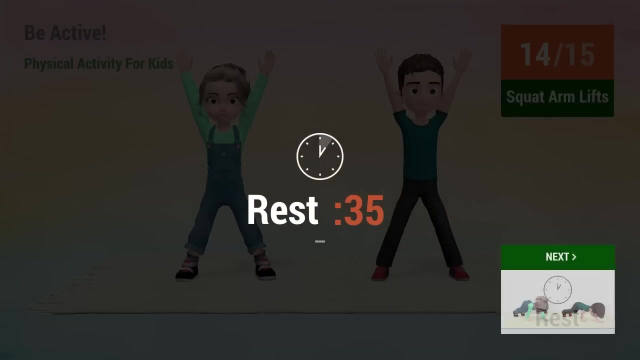 Rest time. Up next squat. Up next squat Squat. arm lifts In: 5,, 4,, 3,, 2,, 1, go 1,, 2,, 3,, 4,, 5,, 6,, 7,, 8,, 9,, 10,, 11,, 12,, 13,, 14, rest time. 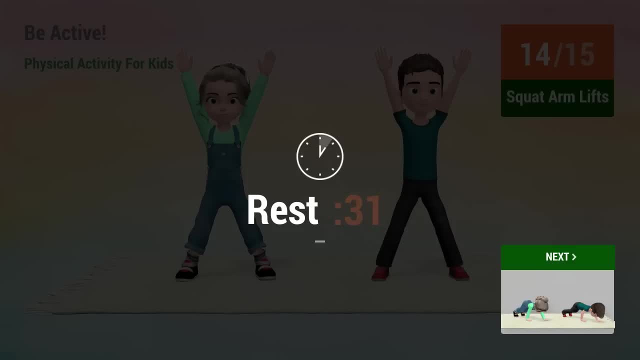 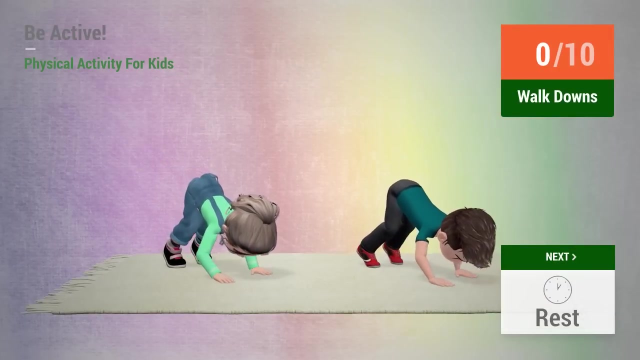 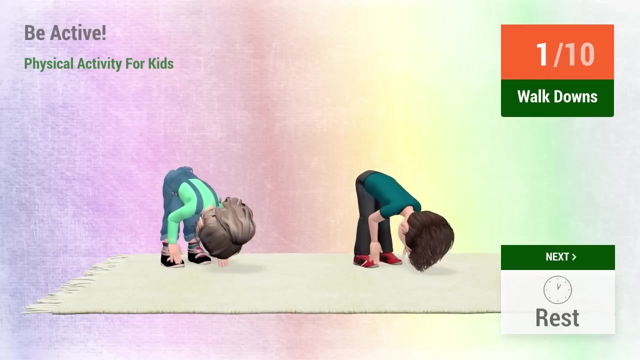 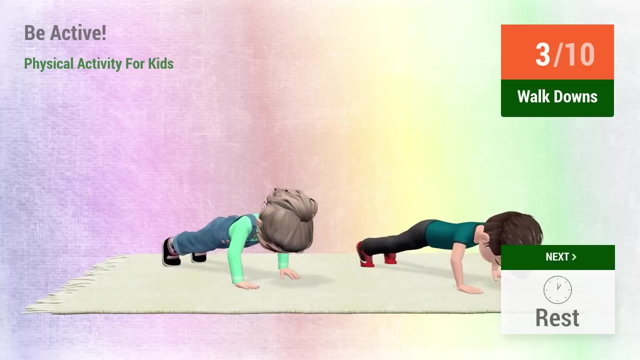 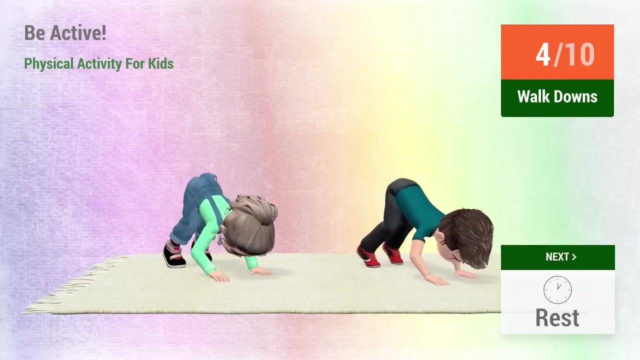 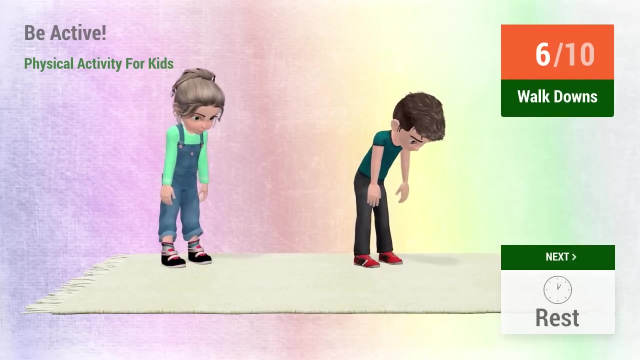 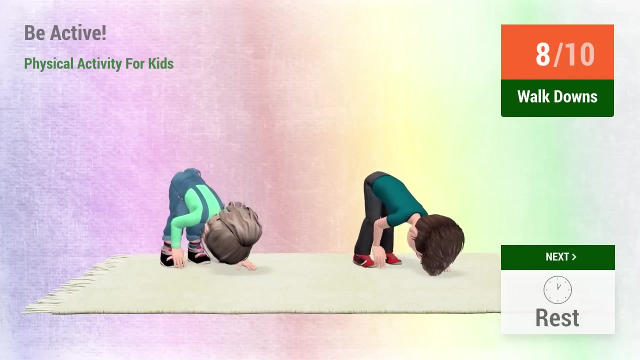 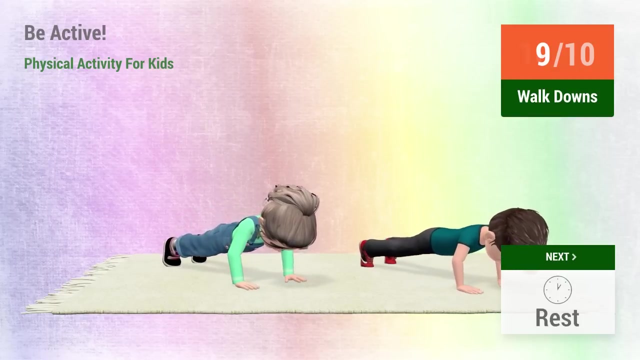 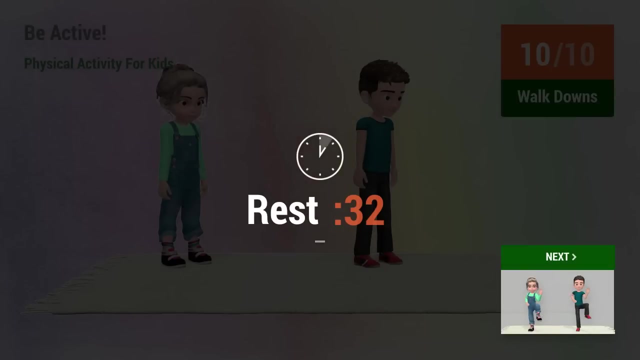 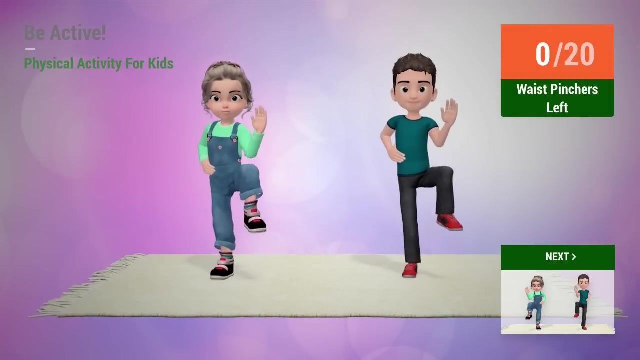 Rest time. up next walk downs in five, four, three, two, one go one, two, three, four, five, six, seven, eight, ten, eleven, twelve, thirteen, fourteen, fifteen, sixteen, twenty, twenty, twenty, thirty, forty, twenty, forty, forty, ninety, twenty, twenty, twenty, thirty, twenty, twenty. up next waist pinchers in five, four, three, two, one. 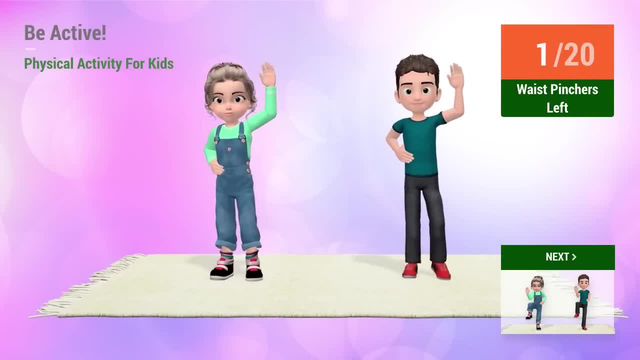 go: 1, 2, 3, 4, 5, 6, 7, 8, 9, 10, 11, 12, 13, 14, 15, 16, 7, 12, 13, 14, 15, 16, 7, 8, 9, 10, 11, 12, 13, 14, 15, 16, 7. 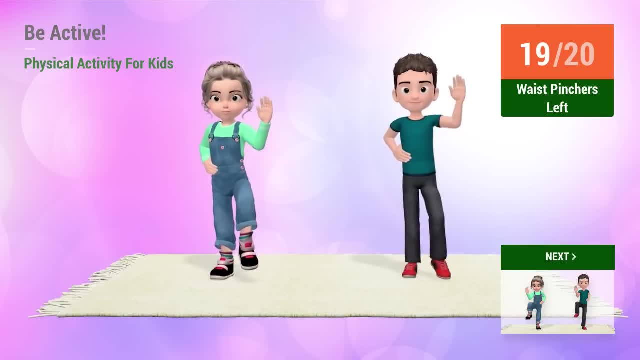 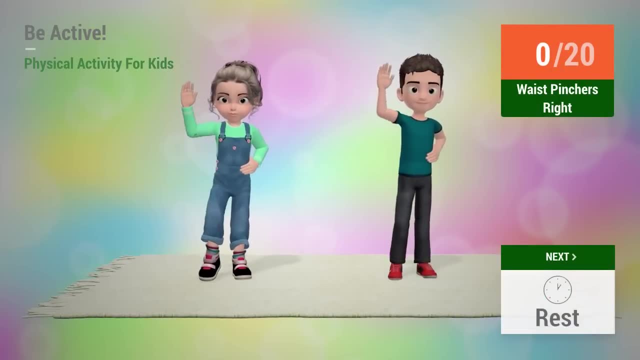 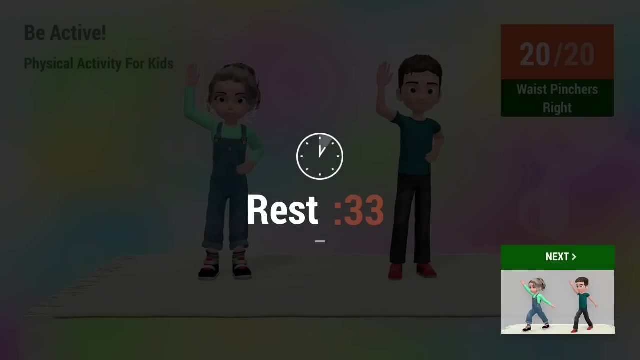 17, 18, 19, 20 up. next waist pinchers in 5, 4, 3, 2. 1. go. 1, 2, 3, 4, 5, 6, 7, 8. go 1, 2, 3, 4, 5, 6, 7, 8, 9, 10, 11, 12, 13, 14, 15, 16, 17, 18, 19, 20 rest time. 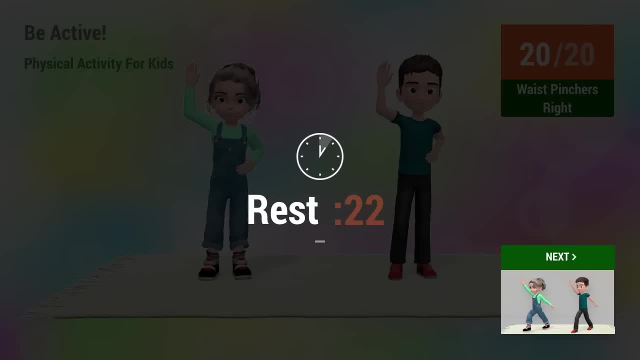 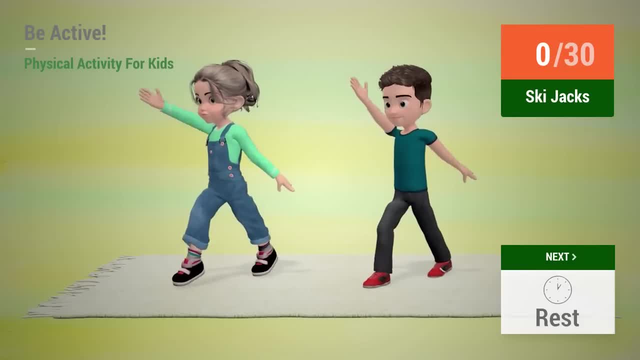 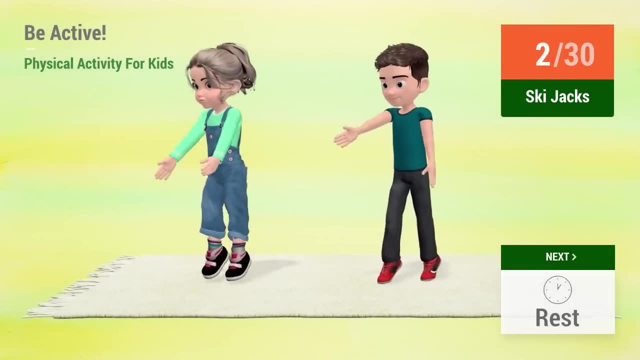 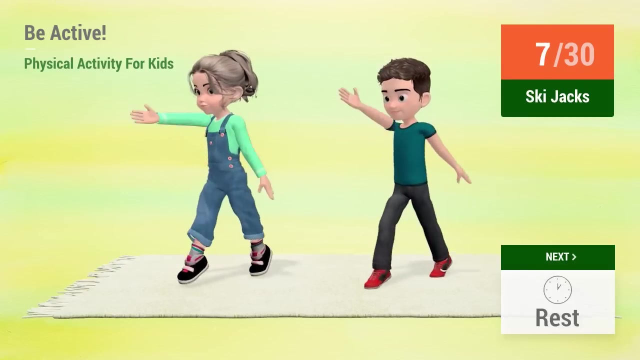 up next sk just with. up next sk just with neem, up next sk just with neem a In 5,, 4,, 3,, 2, 1, go 1,, 2,, 3,, 4,, 5,, 6,, 7,, 8,, 9,, 10,, 11,, 12,, 13,, 14,, 15,, 16,, 17,, 18,, 19,, 20,, 21,. 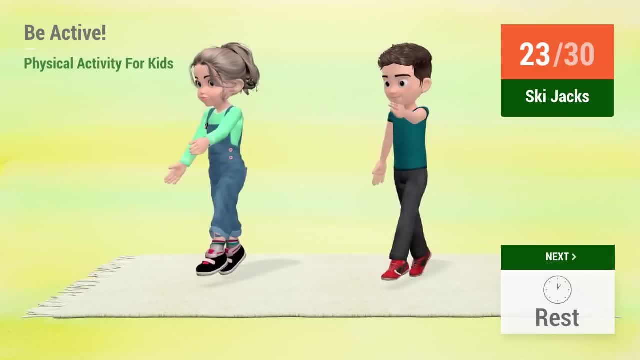 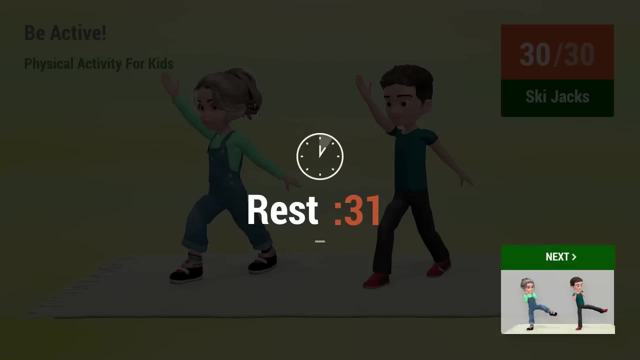 22,, 23,, 24,, 25,, 26,, 27,, 28,, 29,, 30.. Rest time: 1,, 2,, 3,, 4,, 5,, 6,, 7,, 8,, 9,, 10,, 11,, 12,, 13,, 18,, 19,, 20,, 21,, 22,, 23,, 24,, 25,, 26,, 27,, 28,, 30. 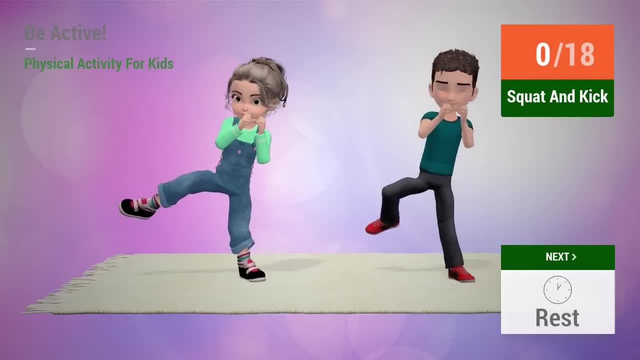 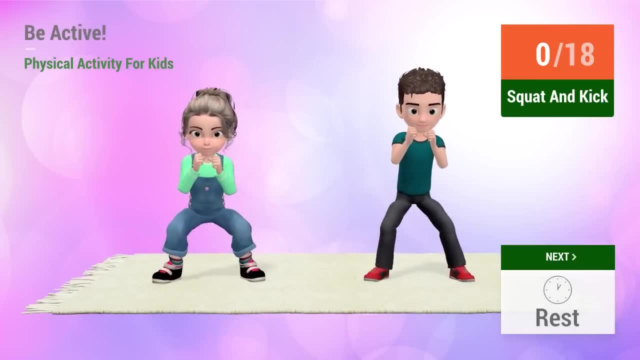 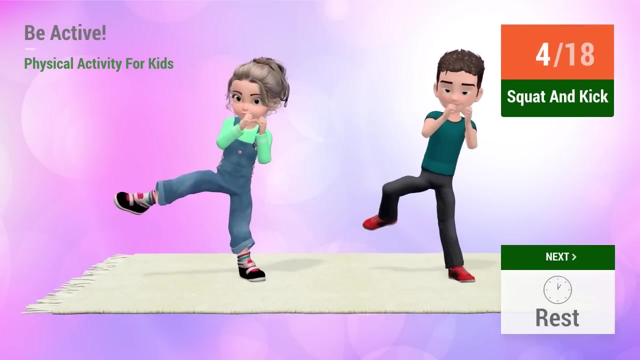 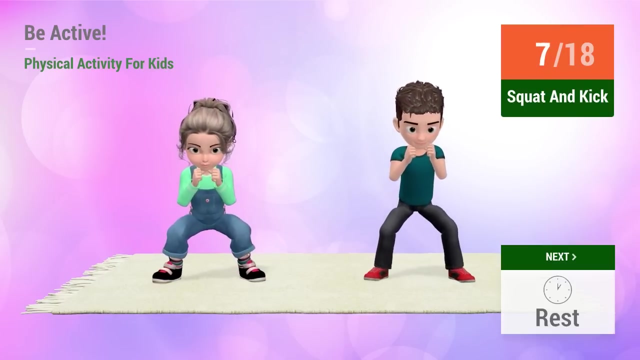 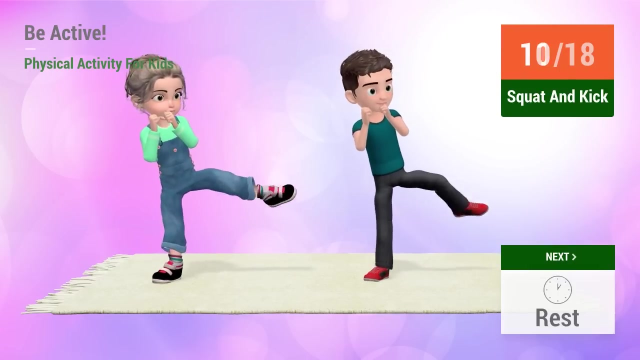 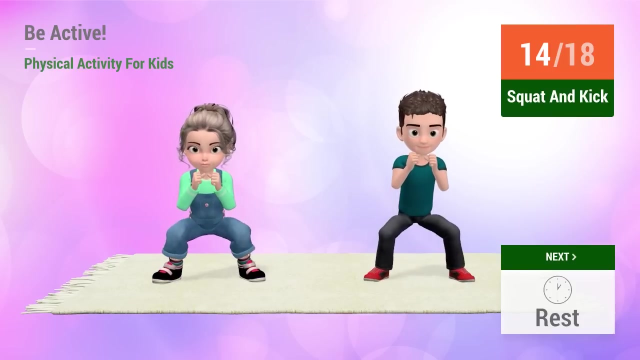 Up next Squat and kick In 5,, 4,, 3,, 2,, 1, go 1,, 2,, 3,, 4,, 5,, 6,, 7,, 8,, 9,, 10,, 11,, 12,, 13,, 14,, 15,. 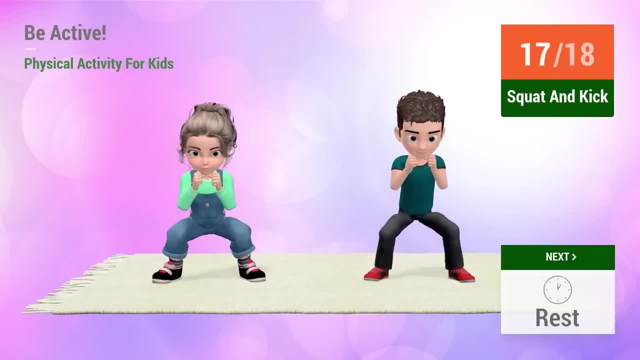 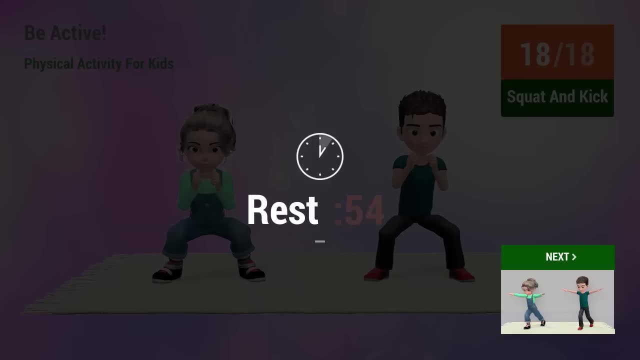 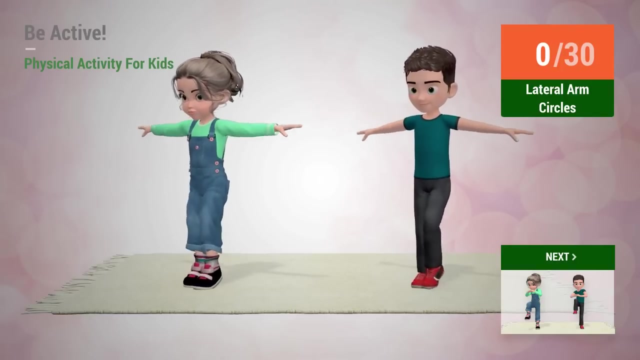 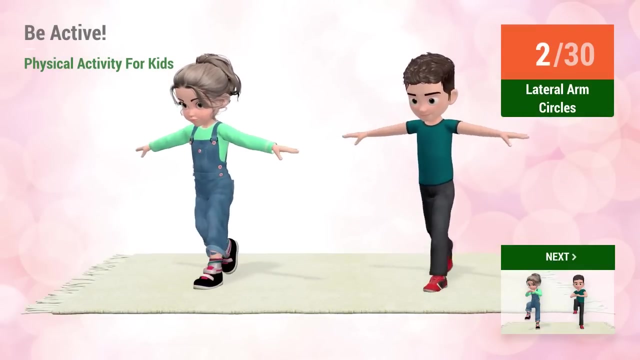 16,, 17,, 18, rest time. Let's go Up next lateral arm circles In 5,, 4,, 3,, 2, 1, go 1,, 2,, 3,, 4,, 5,, 6,, 7,, 8,, 9,, 10,. 11,, 12,, 13,, 14,, 15,, 16,, 17,, 18,, 19,, 20,, 21,, 22,, 23,, 24,, 25,, 26,, 27,, 28,, 29,, 30.. 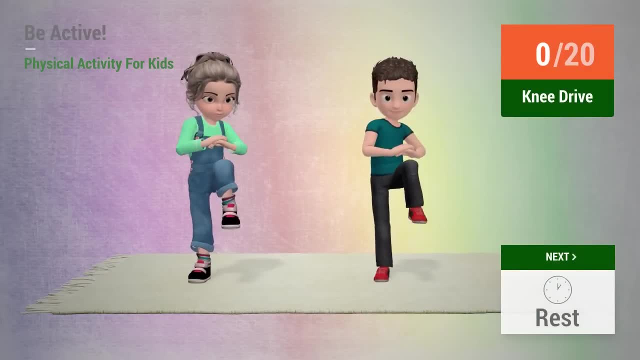 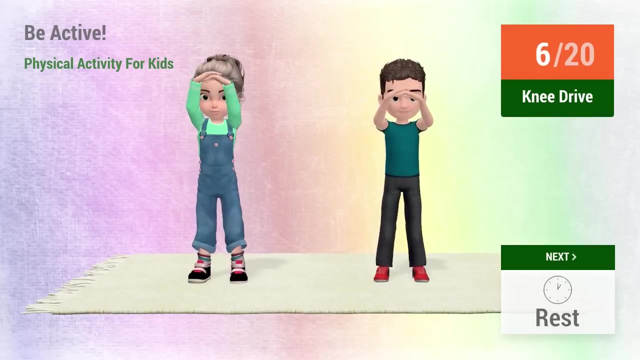 Up next knee, drive In 5.. 4,, 3,, 2,, 1, go 1,, 2,, 3,, 4,, 5,, 6,, 7,, 8,, 9,, 10,, 11,, 12,, 13,, 14,, 15,, 16,, 17,, 18,, 19,, 20, rest time. 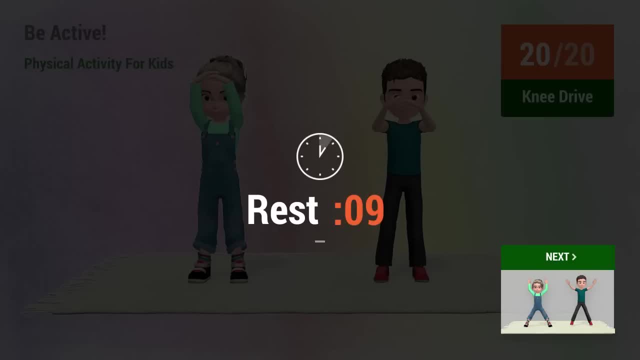 Up next jumping jacks In 5,, 4,, 3,, 2,, 1, go 1,, 2,, 3,, 4,, 5,, 6,, 7,, 8,, 9,, 10,, 11,, 12,, 13,, 18,, 19,, 20,, 21,, 22,, 23,, 24,, 25,, 26,, 27,, 28,, 29,, 30. In 5,, 4,, 3,, 2,, 1, go 1,, 2,, 3,, 4,, 5,, 6,, 7,, 8,, 9,, 10,, 11,, 12,, 23,, 24,, 25,, 26,, 29,, 30. In 5,, 4,, 3,, 2,, 1, go 1,, 2,, 3,, 4,, 5,, 6,, 7,, 8,, 9,, 10,, 11,, 12,, 23,, 24,, 25,, 26,, 29,, 30. 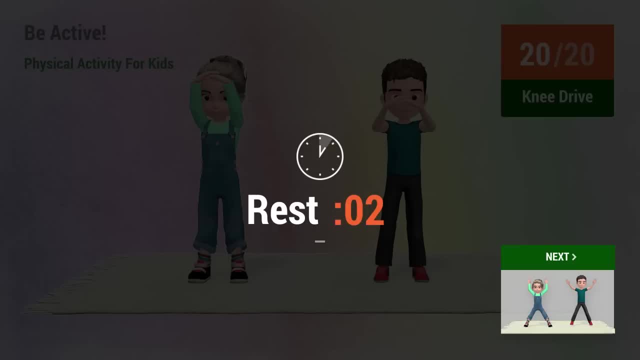 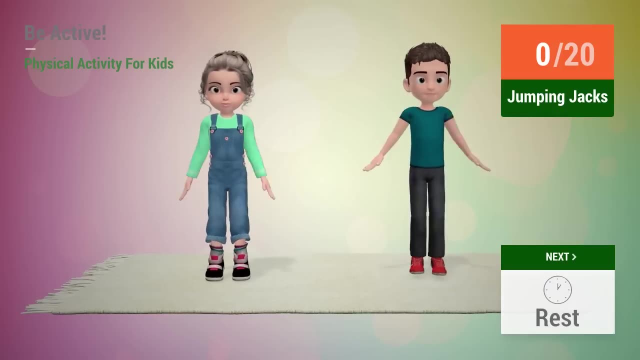 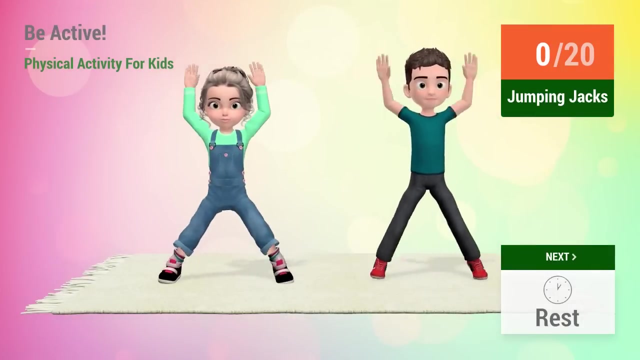 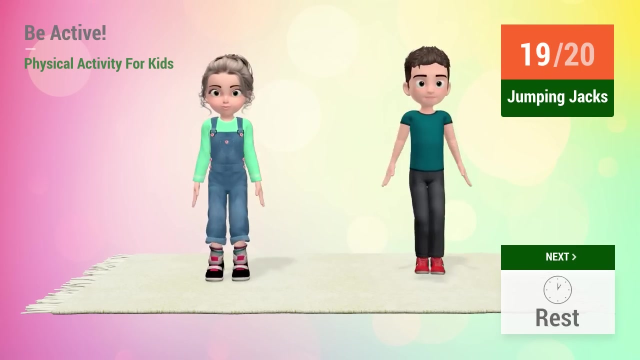 In 5,, 4,, 3,, 2,, 1,. go up next jumping jacks in five, four, three, two, one. go one, two, three, four, five, six, seven, eight, nine, ten, eleven, twelve, thirteen, fourteen, fifteen, sixteen, 17, 18, 19, 20 rest time. 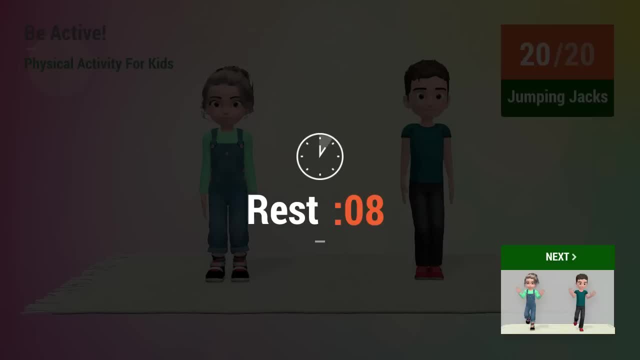 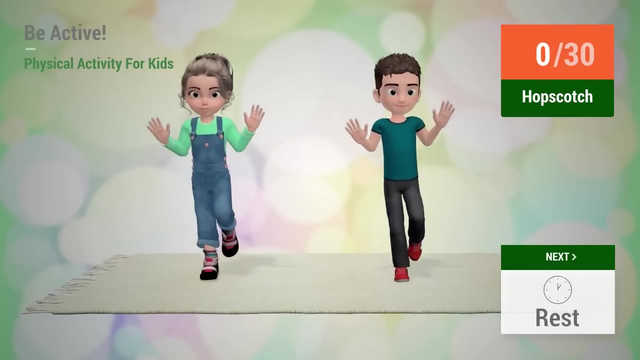 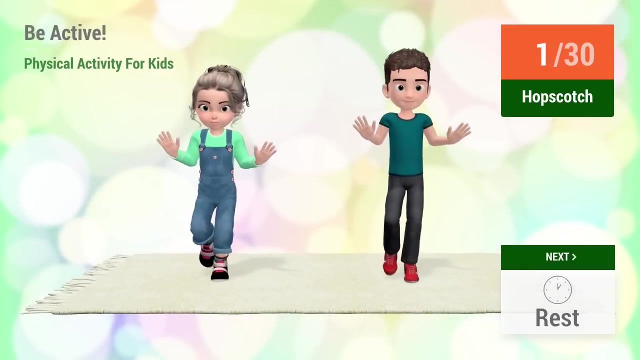 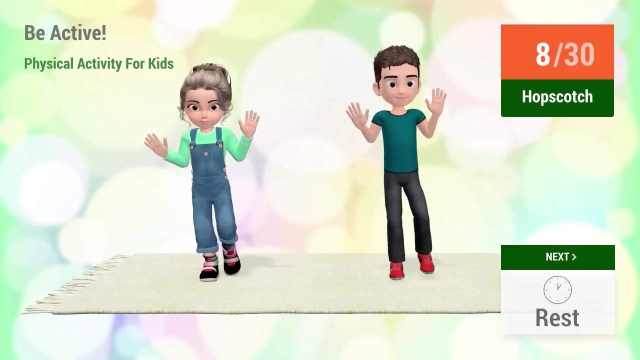 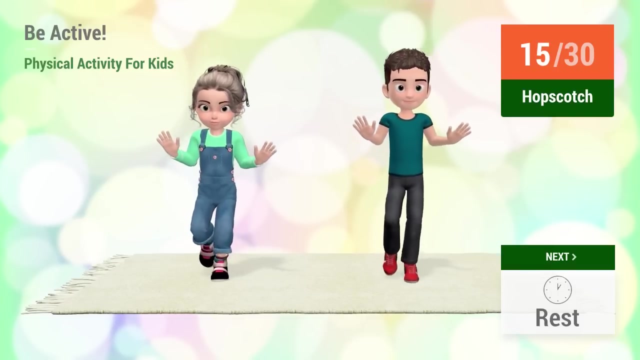 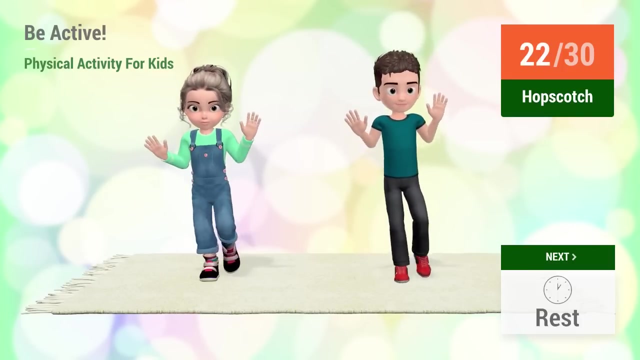 up next hopscotch in five, four, three, two, one go one, two, three, four, five, six, seven, eight, nine, ten, eleven, twelve, thirteen, fourteen, fifteen, sixteen, 17, 18, 19, 20, 21, 22, 23, 24, 25, 26, 27, 28, 29, 30 rest time. 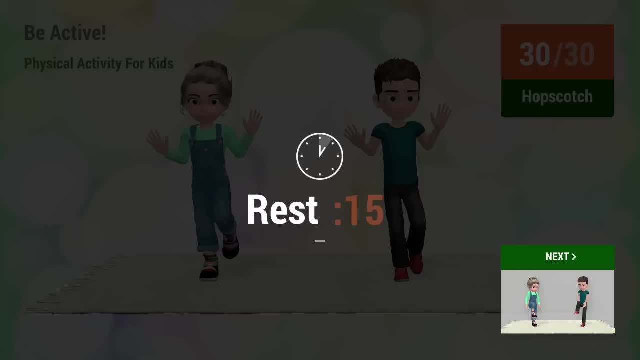 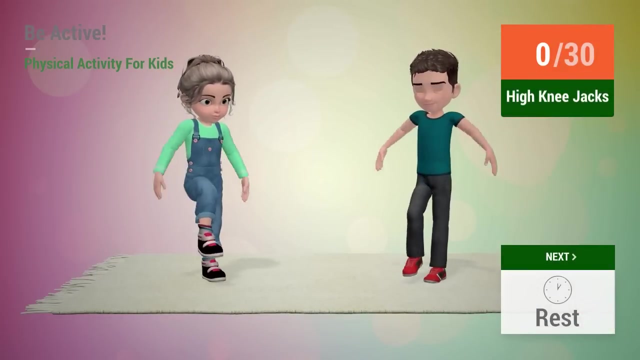 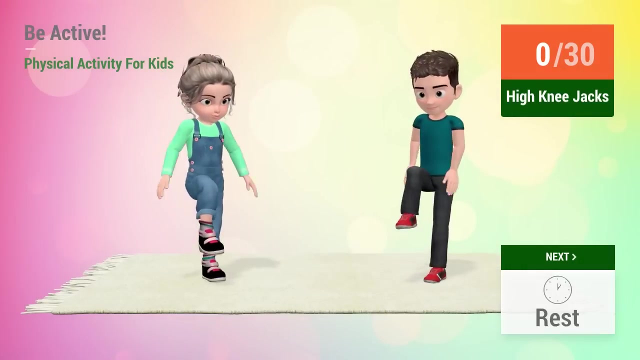 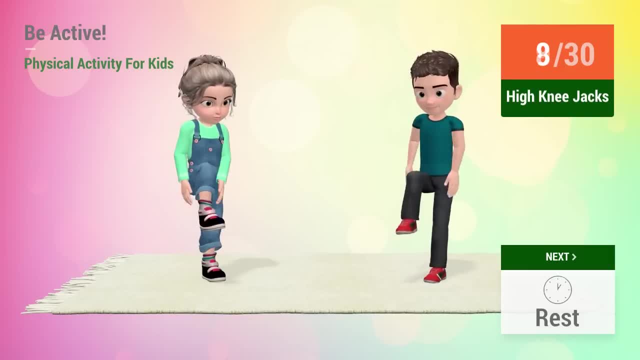 up next high knee jacks in five, four, three, two, one go one, two, three, four, five, six, 7, 8, 9, 10, 11, 12, 13, 14, 15, 16, 17, 18, 19, 20, 21, 23. 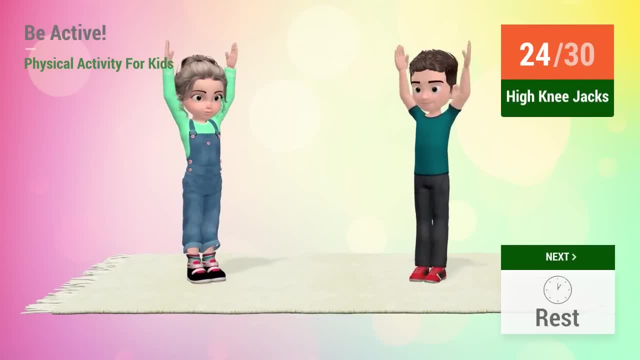 up next high knee jacks in five, four, three, two, one, two, three, four, five, six, 7, 8, 9, 10, 12, 13, 16, 17, 18, 19, 20, 23, 24, 25, 26, 27, 28, 29, 30 rest time. 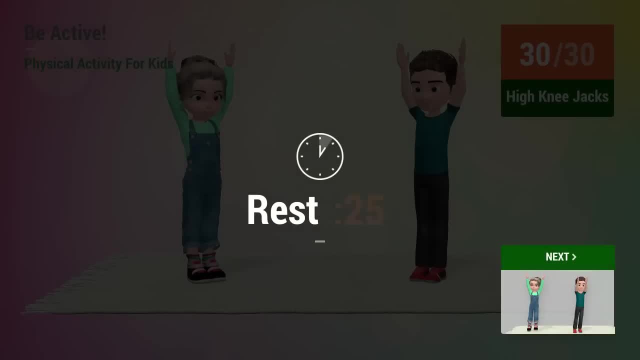 up next high knee jacks in five, four, three, two, one, two, three, four, five, six, 7, 8, 9, 10, 12, 13, 16, 17, 18, 19, 20, 23, 24, 25, 26, 27, 28, 29, 30 rest time. 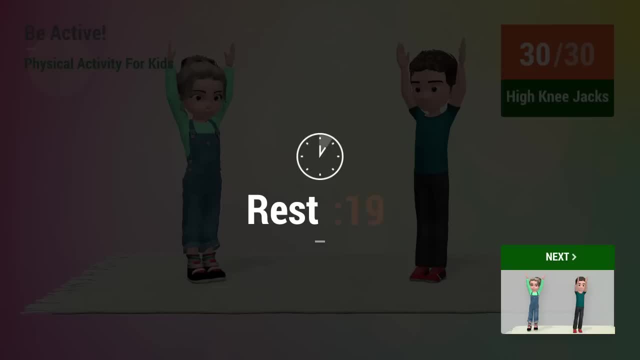 up next high knee jacks in five, four, three, two, one, two, three, four, five, six, 7, 8, 9, 10, 12, 13, 16, 17, 18, 19, 20, 23 rest time. up next high knee jacks in five, four, three, two, one, two, three, four, five, six, 7, 8, 9, 10, 12, 13, 16, 18, 19, 20, 23 rest time. 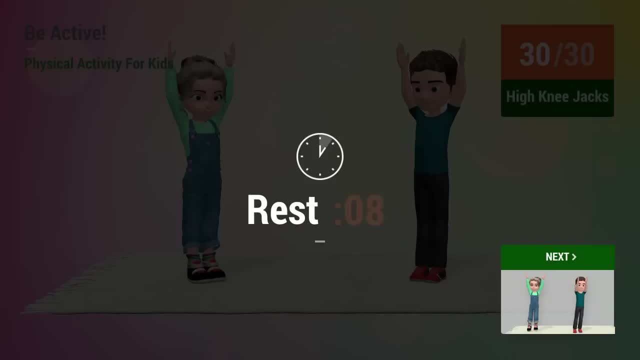 up next high knee: jacks in five, four, three, two, one, two, three, four, five, six, 7, 8, 9, 10, 12, 13 rest time. up next high knee: jacks in five, four, three, two, one, two, three, four, five, six, 7, 8, 9, 10, 12, 13, 16, 18, 19, 20, 23 rest time. 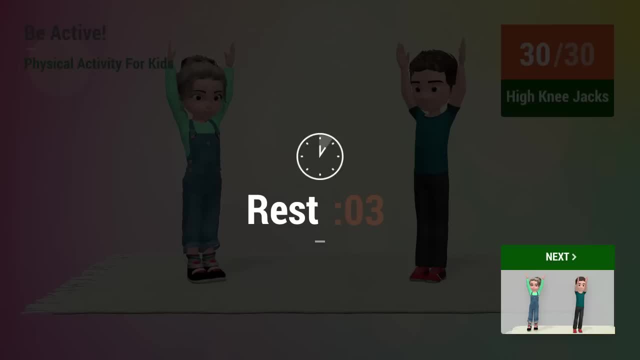 up next high knee jacks in five, four, three, two, one, two, three, four, five, six, 7, 8, 9, 10, 12, 13, 16, 18, 19, 20, 23 rest time. up next high knee jacks in five, four, three, two, one, two, three, two, one, two, three, four, five, six, 7, 8, 9, 10, 12, 13, 16, 18, 19, 20, 23 rest time. 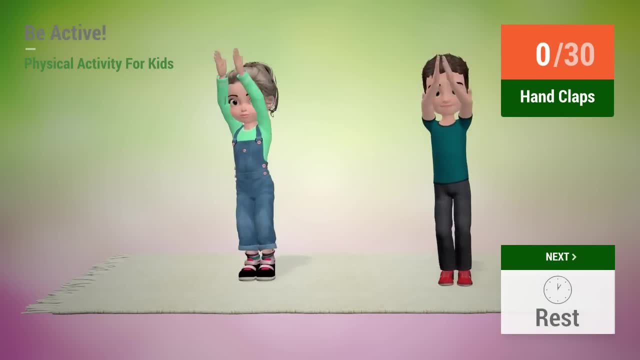 up next high knee jacks in five, four, three, two, one, two, three, two, one, two, three, four, five, six, 7, 8, 9, 10, 12, 13 rest time. up next high knee jacks in five, four, three, two, one, two, three, two, one, two, three, four, five, six, 7, 8, 9, 10, 12, 13 rest time. 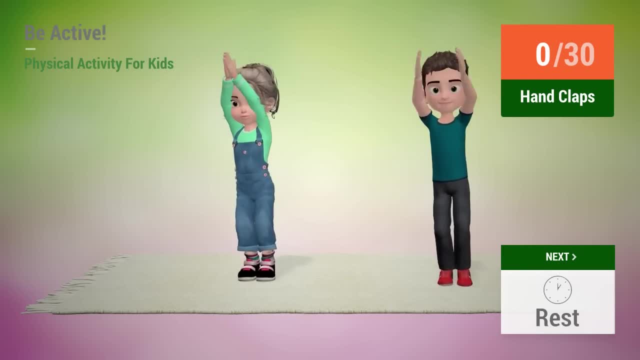 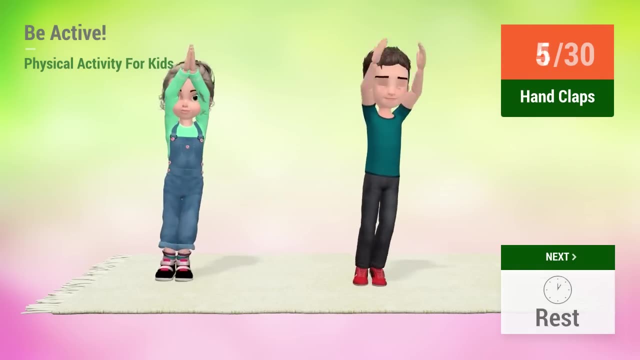 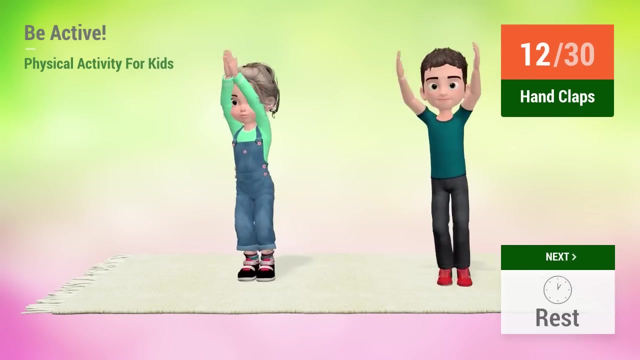 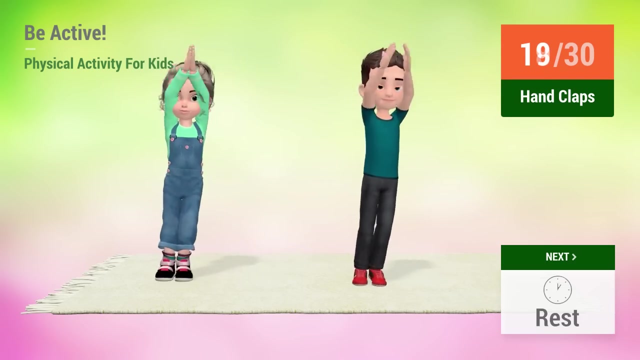 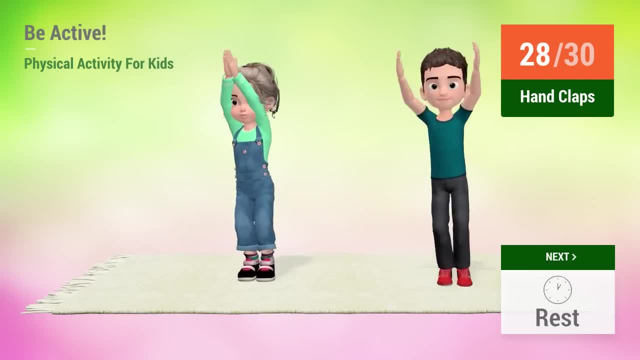 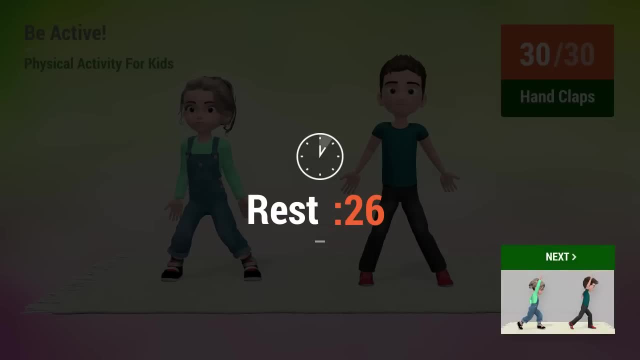 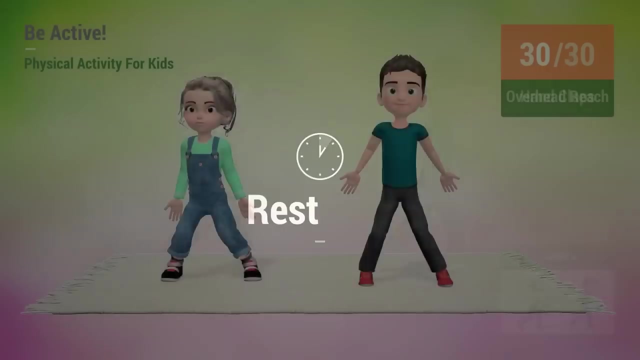 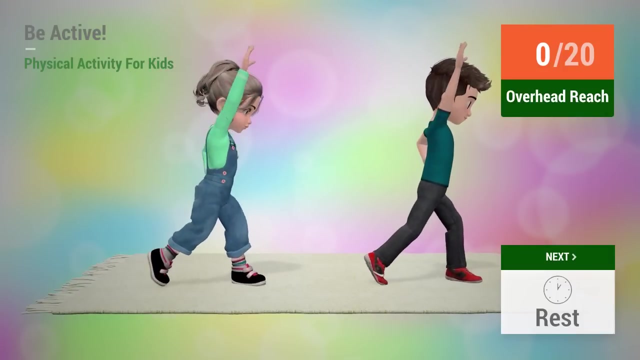 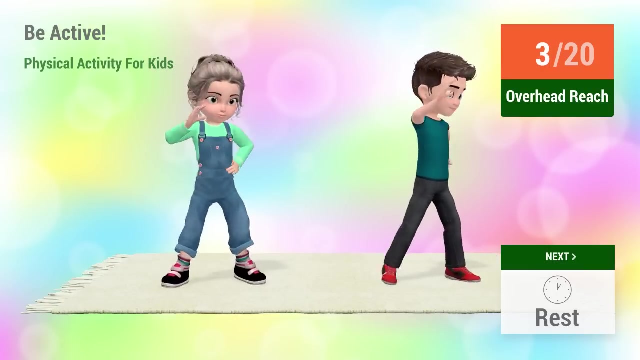 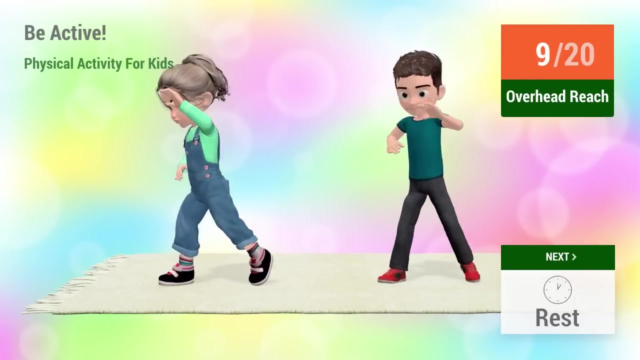 25,, 26,, 27,, 28,, 29,, 30 Rest time. Up next overhead reach In 5,, 4,, 3,, 2, 1, go 1,, 2,, 3,, 4,, 5,, 6,, 7,, 8,, 9,, 10. 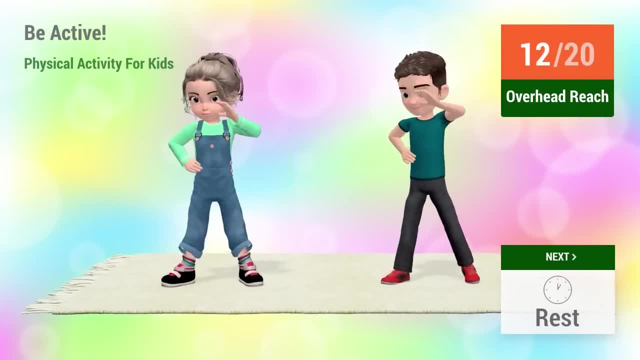 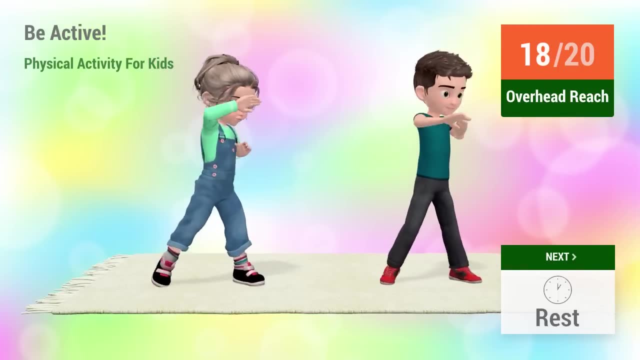 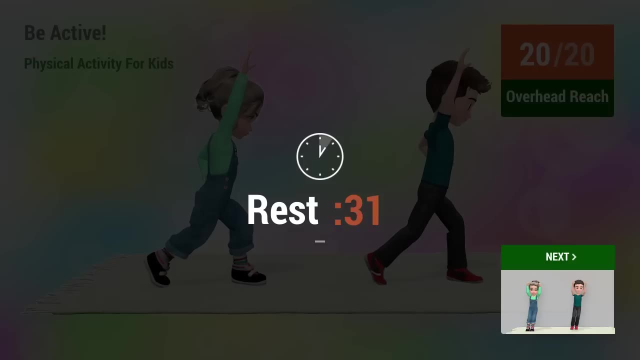 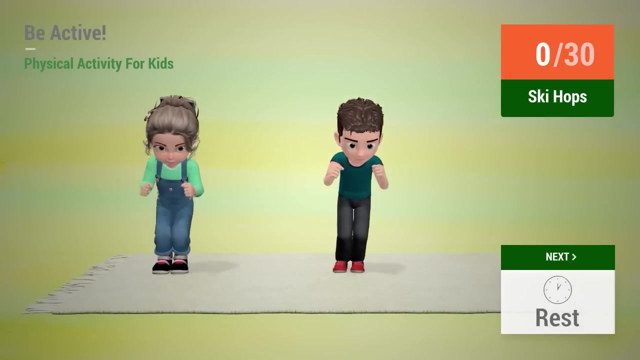 10,, 11,, 12,, 13,, 14,, 15,, 16,, 17,, 18,, 19,, 20 Rest time. Up next ski hops In 5,, 4,, 3,, 2,, 1, go. 1,, 2,, 3,, 4,, 5,, 6,, 7,, 8,, 9,, 10, 11,, 12,, 13,, 14,, 15,, 16,, 17,, 18,, 19, 20. 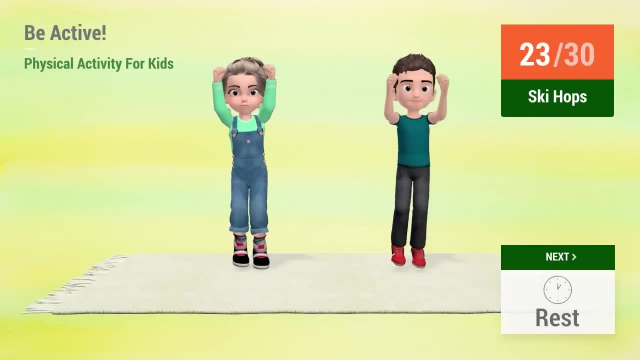 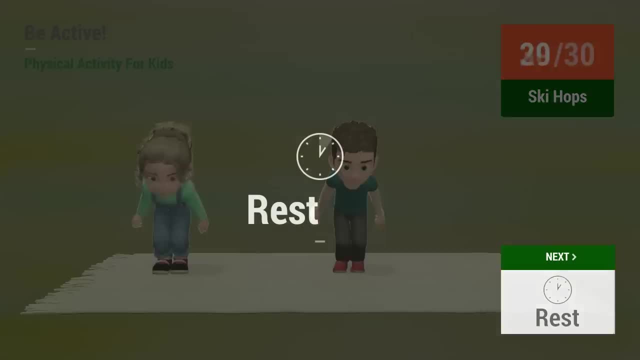 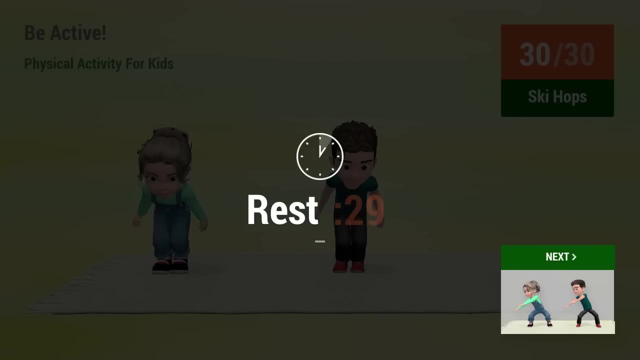 21,, 22,, 23,, 24,, 25,, 26,, 27 Rest time, 28,, 29,, 30 Rest time 30,, 31,, 32,, 33,, 34,, 35,, 36,, 37,, 38,, 39,, 40. 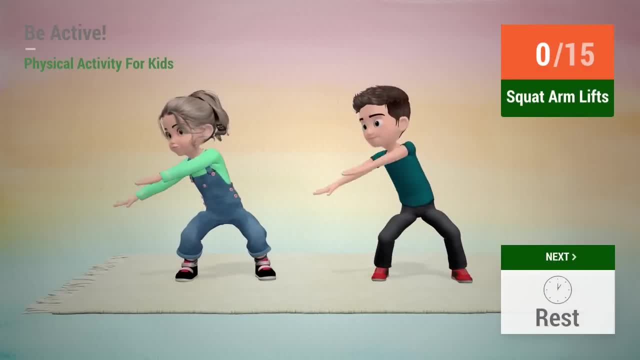 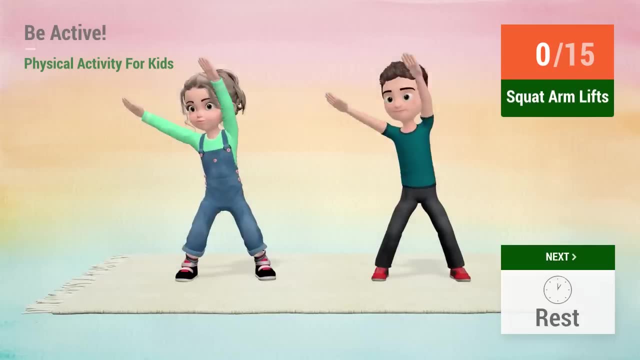 Up next squat arm lifts In 5,, 4,, 3,, 2, 1, go 1,, 2,, 3,, 4,, 5,, 6,, 7,, 8,, 9,, 10,, 20. 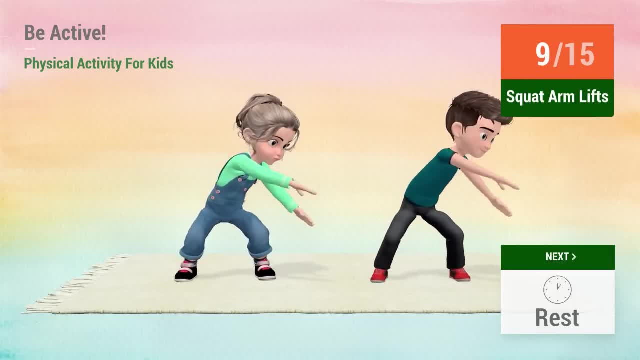 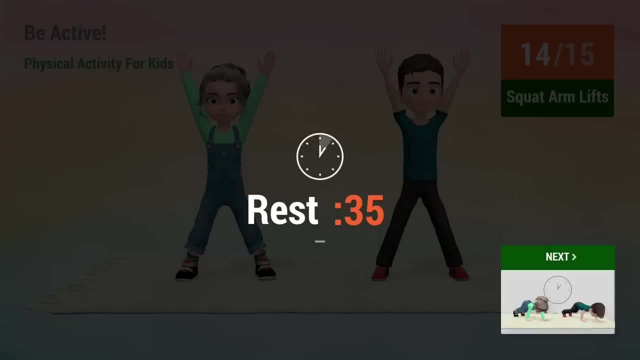 1,, 2,, 3,, 4,, 5,, 6,, 7,, 7,, 8,, 9,, 10,, 11,, 12,, 13, 14 Rest time. Rest time Up. next walk-downs. 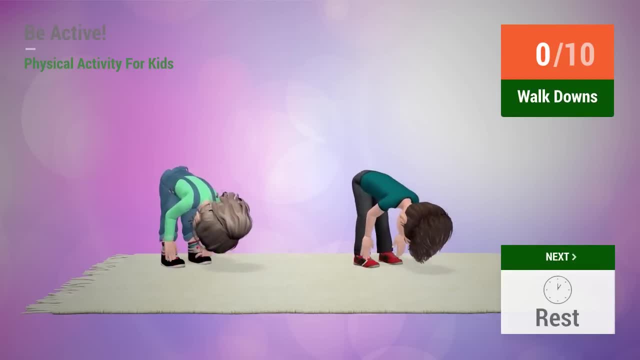 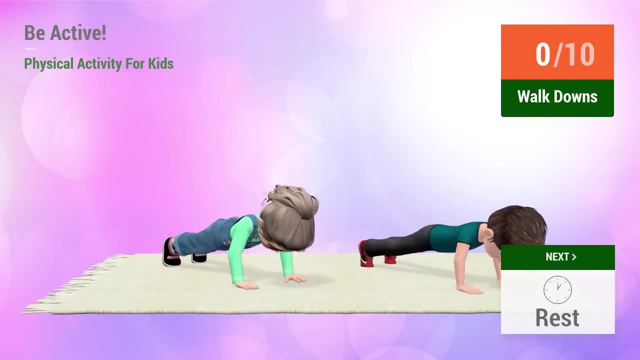 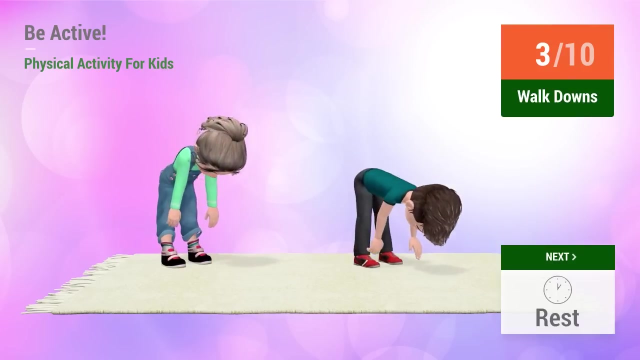 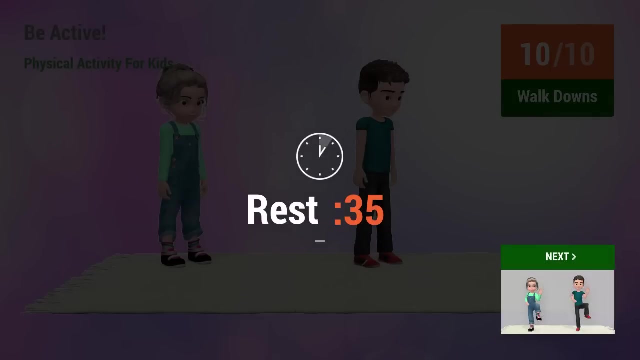 In 5,, 4,, 3,, 2,, 1, go 1,, 2,, 3,, 4,, 5,, 6,, 7,, 8,, 9,, 10. Rest time. 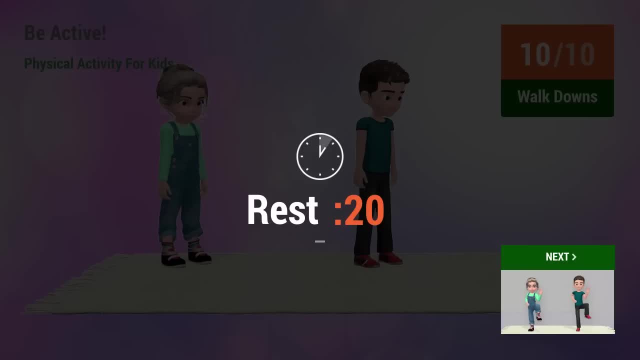 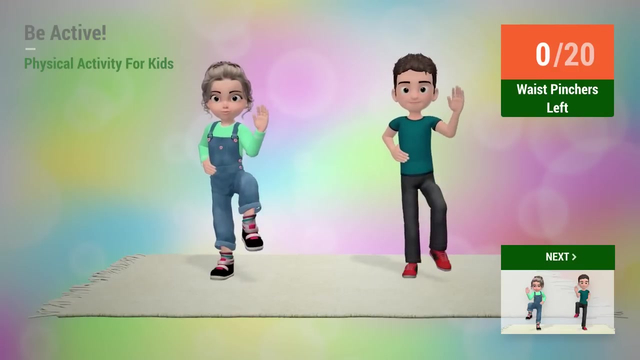 Up next waist pinchers In 5,, 4,, 3,, 2,, 1, go 1,, 2,, 3,, 4,, 5,, 6,, 7,, 8,, 9,, 10,, 11,, 12,, 13,, 14,, 15,, 16,, 17,, 18,, 19,, 20,, 21,, 22,, 23,, 24,, 25,, 26,, 27,, 28,. 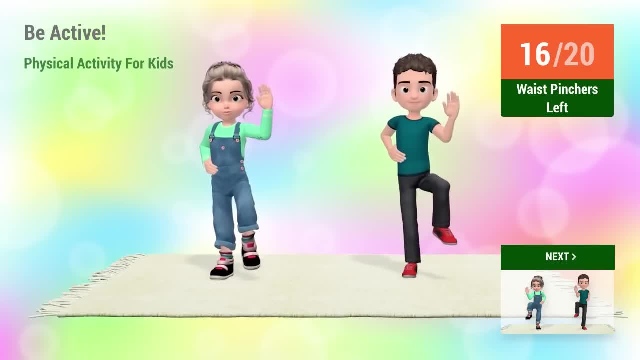 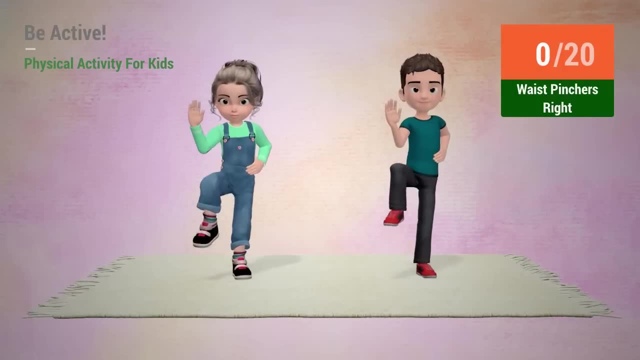 28,, 29,, 30,, 31,, 32,, 34,, 35,, 36,, 37,, 38,, 39,, 40,, 41,, 42,, 43,, 45,, 41,, 42,, 44,, 43,, 45,, 45,, 46,, 47,, 49,, 50,, 51,, 42,, 43,, 45, 46, COVID 46,, 49,, 42,, 45,, 47,, 49,, 40,, 42,, 45,, 40,, 42,, 42,, 42,, 43,, 43,, 44,, 45,, 44,, 46,, 46,, 47,, 47,, 49,, 51,, 42,, 43,, 44,, 45,, 46,, 47,, 50,, 42,, 48,, 42,, 44,, 45,, 46,, 47,, 48,, 49,, 50,, 52,, 53,, 54,, 56,, 49,, 51,, 52,, 53,, 54, Gr posture ornamental نے Operations.